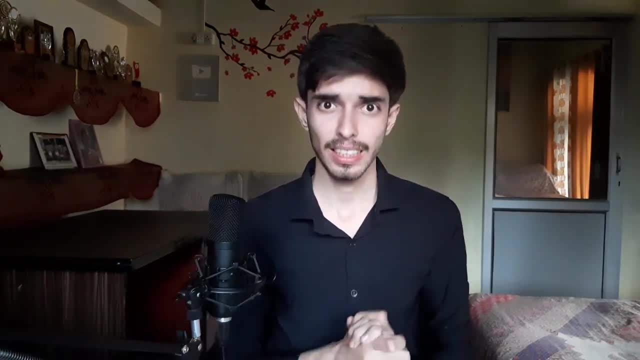 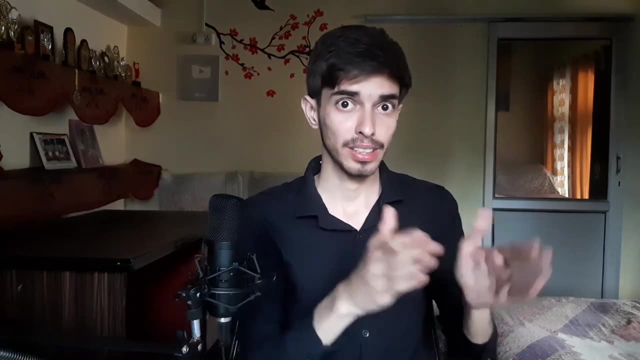 calendar and it started with the sunday. okay, clear. so for any date from that day we can calculate how many whole weeks were passed, like 7, 7, 7, 7, 7, and then how many extra days are passed, and those extra days are the number of odd days. so that's the number of odd days and that's the number of. 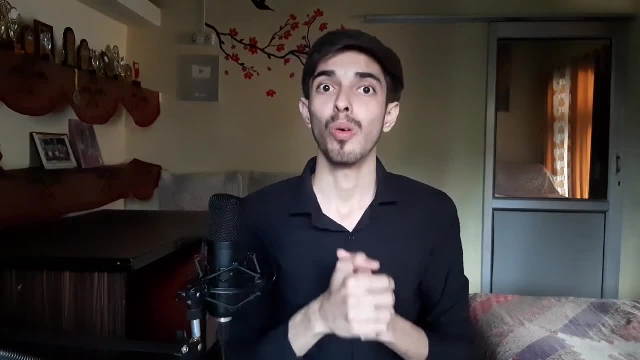 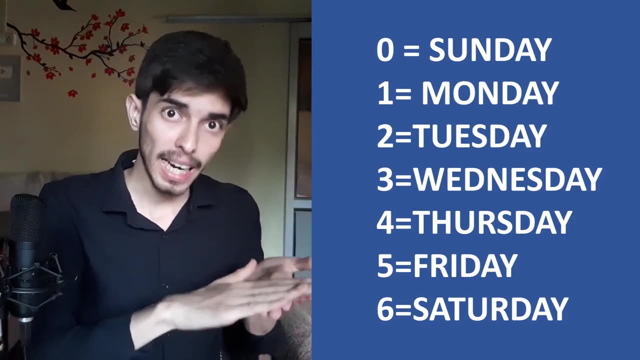 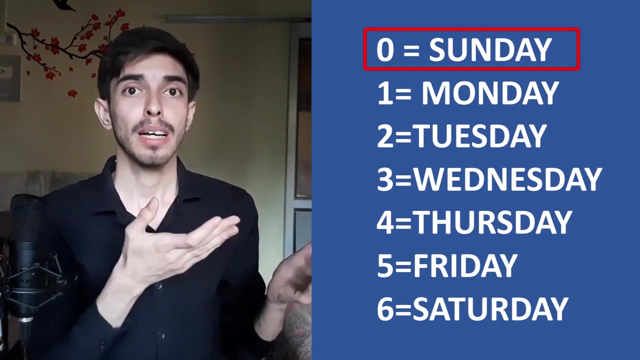 other days of the weeks. okay, so that is called the odd days. so simply odd days, the number from zero to six. so if zero or days are passed for a certain date, then on that certain date it is a sunday, okay. and for example, if four odd days are passed, then it is a thursday, okay. so it is simple. 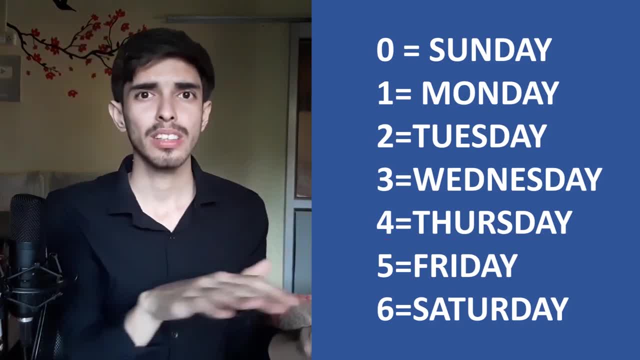 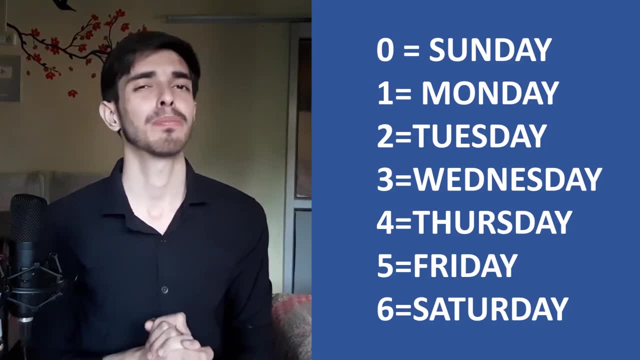 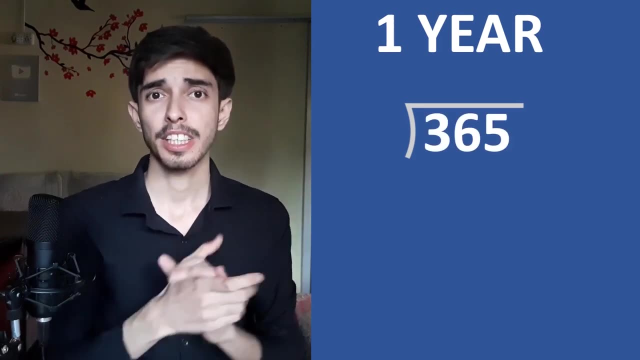 we are just starting from sunday and calculating all the way till that day and seeing how many days are passed, and that odd day number gives us the day of the week. as simple as that. okay, so i have a question for you. calculate the odd days for one year, that is, 365 days. c divide by 7, as 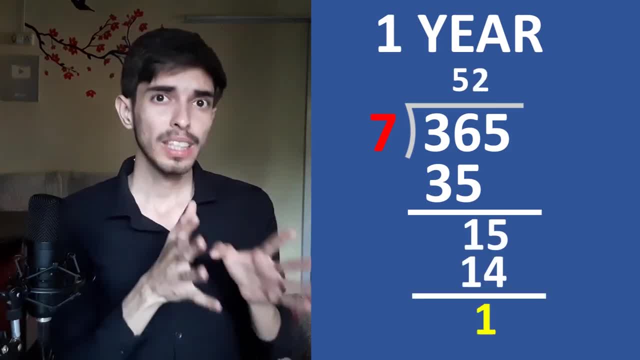 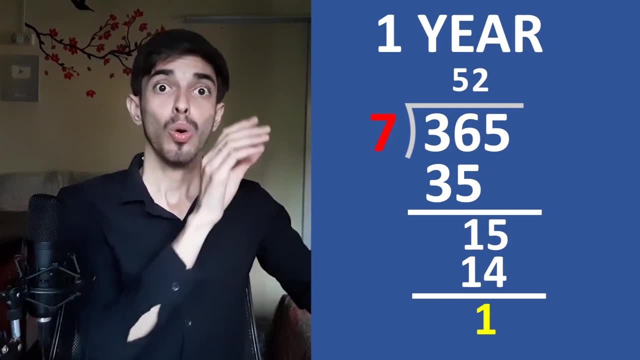 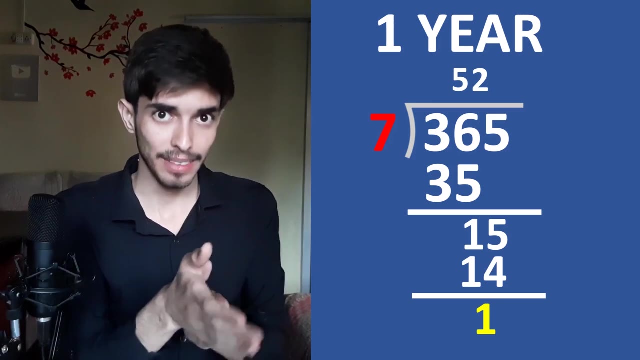 simple as that. and c- remainder. remainder is 1, so one odd day. this means that, for example, on a certain date on this year it is a monday. on that same certain date on the next year it will be a. so there is a difference of one extra day. so this was for a normal year. what happens for a leap year? 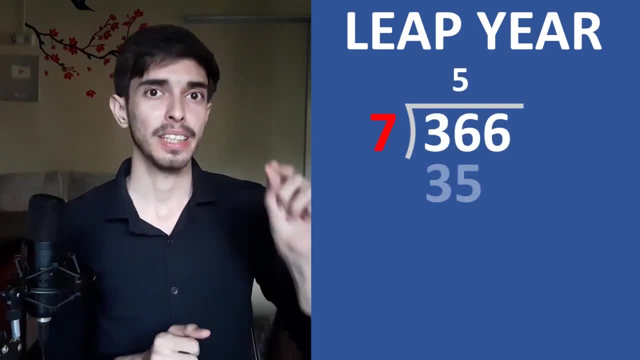 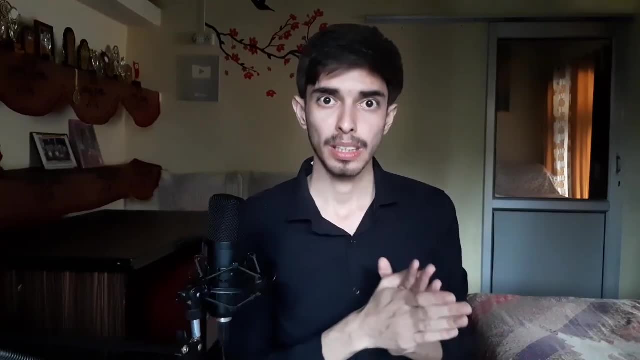 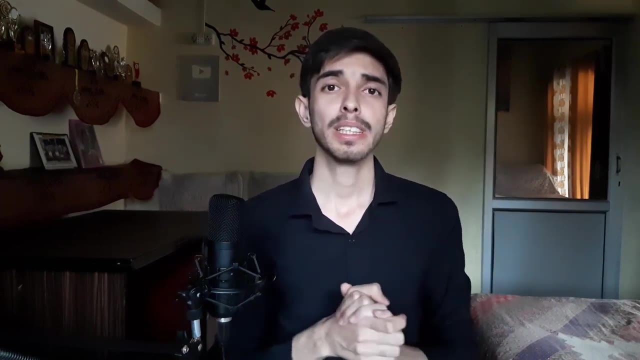 366 days. divide by 7, remainder is 2, so there is a lead of 2 days whenever a leap year passes. so you have to remember this: whenever a year passes one odd day and whenever a leap year passes two odd days. as simple as that. so, with this information, tell me the odd days when 100 year passes. it is. 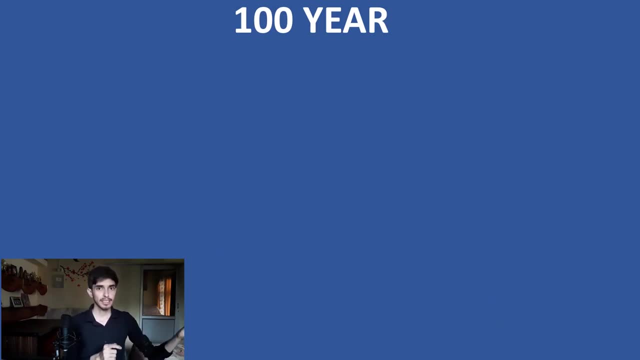 extremely simple to do, see. we need to find how many leap year passes and how many normal year passes from there, calculate their odd days and then so on. we will get our answer. let us do it see: 100 divided by 4, we get 25 and remainder 0. so 25 leap years are there in a 100 year, right? no, 100 is not a leap. 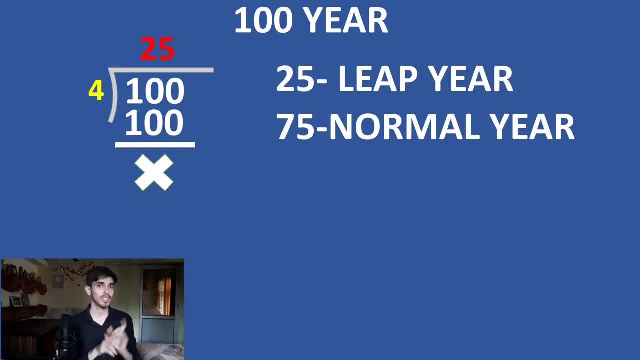 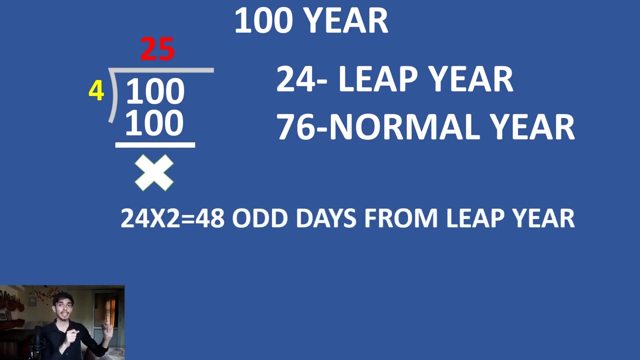 year, it should be divisible by 402, which is not okay. so there are 24 leap years in 100 year and 20 normal years. so with this we have 48 odd days from leap year, because every leap year have two odd days and 76 odd days from normal years. now we will simply add this, we will get 124, so 124. 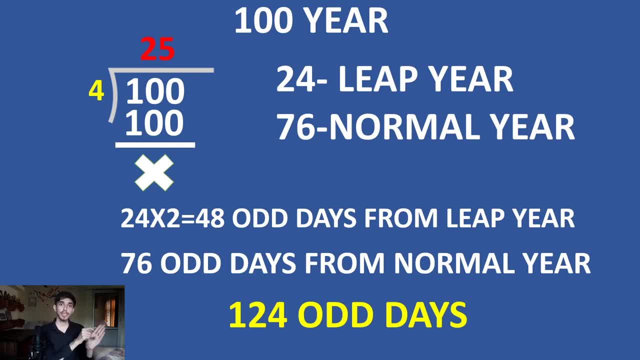 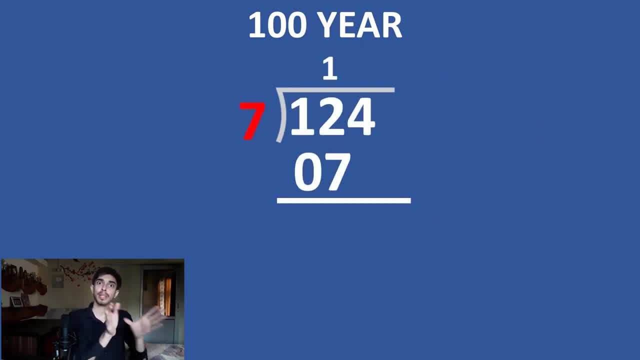 odd days. now the odd day number should be 0 to 6. okay, so whenever there is more divide by 7- because these days are also making up weeks, okay, so they tend to be divided by 7 into weeks and so on. so together come up and neutralize that lag. so that is why we are dividing it by seven- we get a. 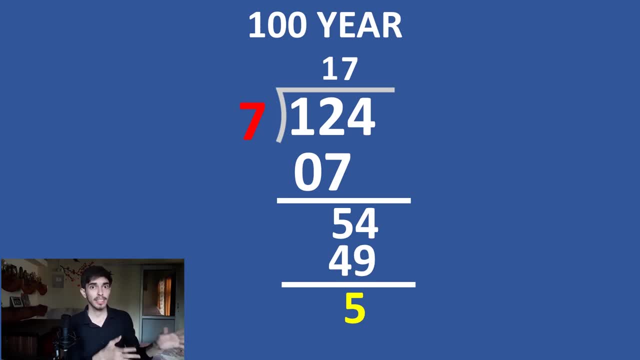 remainder of five. so whenever a hundred year passes, we get a lead, or we can also say a lag, of five days. okay, so for 100 year we have five odd days for 200 years. see, it is extremely simple: for 100 years we have five, for 200 years, another five, so 10, which is bigger than six. divide by 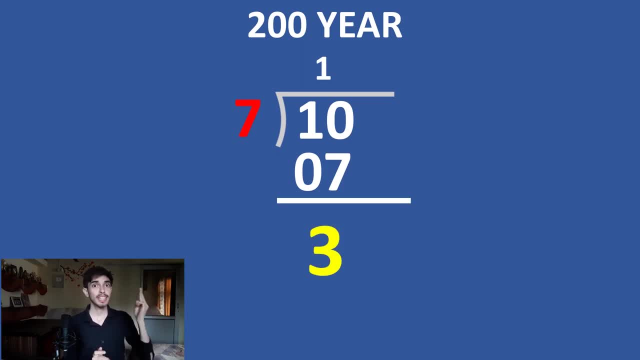 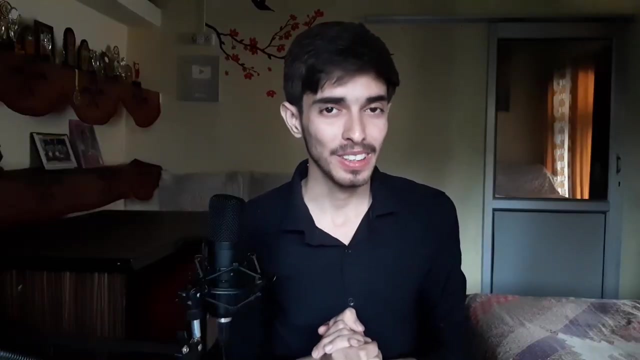 seven, we get a remainder of three. so for every 200 year we have three odd days. now for 300 year, similarly: 15 divide by seven, remainder one, one odd day. now tell me, for 400 years, simple, 20 divide by seven, we get a remainder of six. so six odd days. now it is wrong because see, 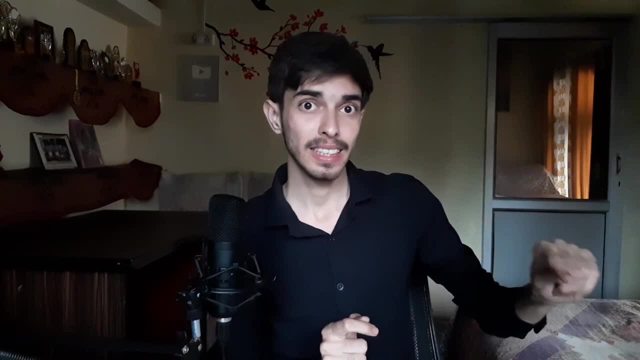 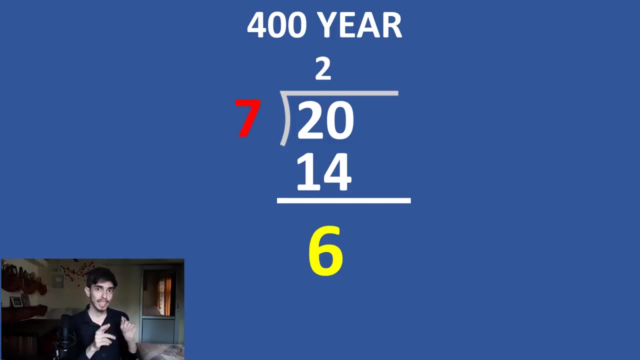 in calculating for 100, 200, 300, we didn't consider them as leap year, but we have to consider 400 as a leap year. so 21 odd days, because that leap year will give one extra odd days. so 21 odd days and 21 divided by seven, with a remainder of zero, that means 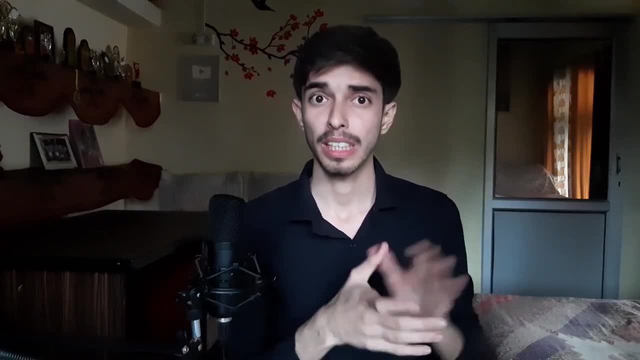 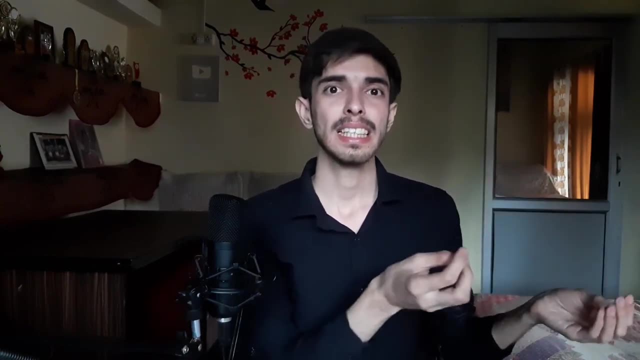 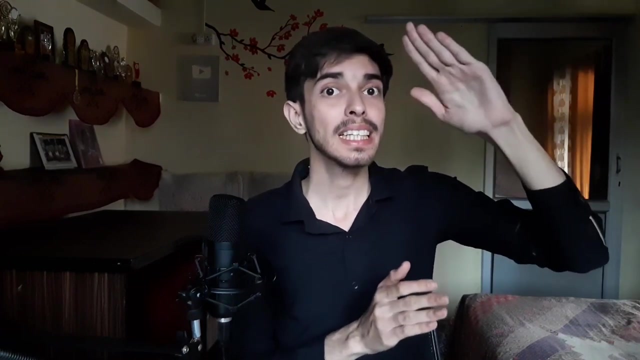 zero odd days. so this gives us a extremely important information. that is, the gregorian calendar resets every 400 years, so normally we get dates in 1800s, 1900s, etc. so we will start from 1600 because on 1600 the gregorian calendar reset. okay, so we won't start from one date of. 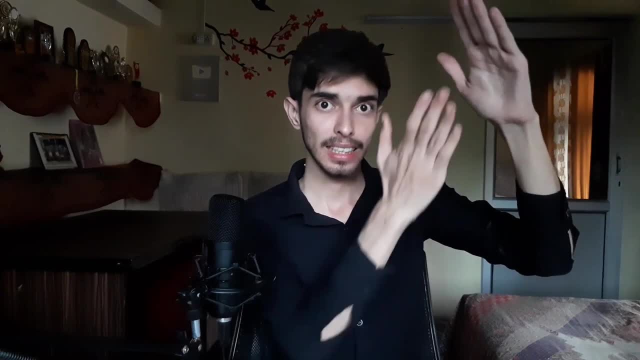 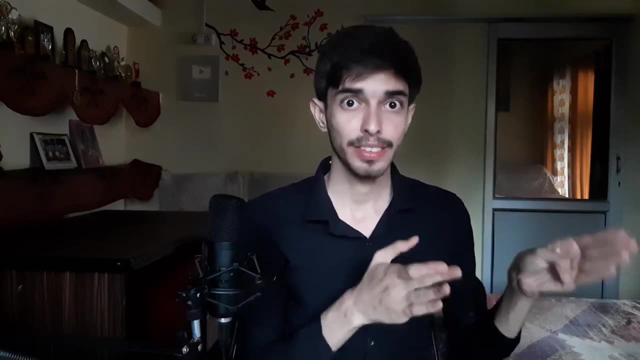 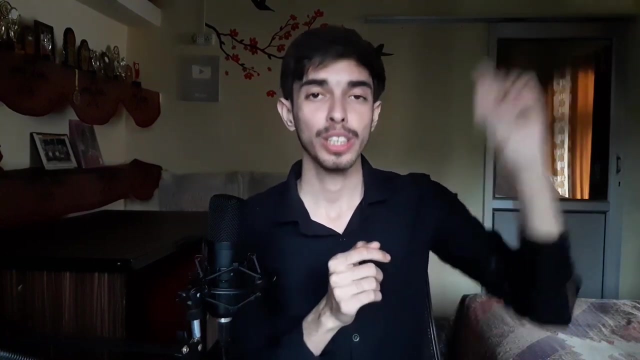 gregorian calendar we will start from 1600 year and then go to our date to find the day of the week, okay, and remember. for finding odd days, we divide by seven and check for remainder. for finding leap years, we divide by four and look at the quotient and also keep in mind that other condition of leap 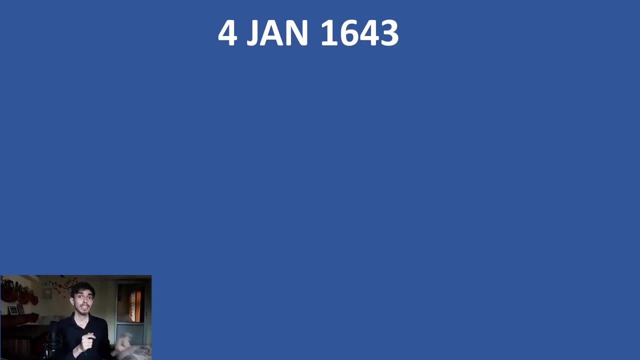 two. now let's solve a question on this. tell me the day of the week on for january 1643. this is the date of birth of sir isaac newton, according to the gregorian calendar. on internet you will find another date too. that is from julian calendar, and we work with only gregorian calendar. okay, so see. 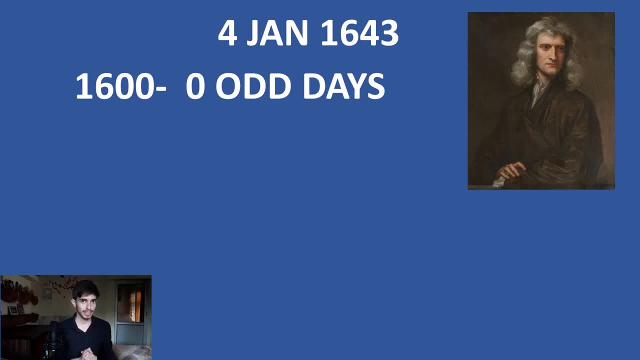 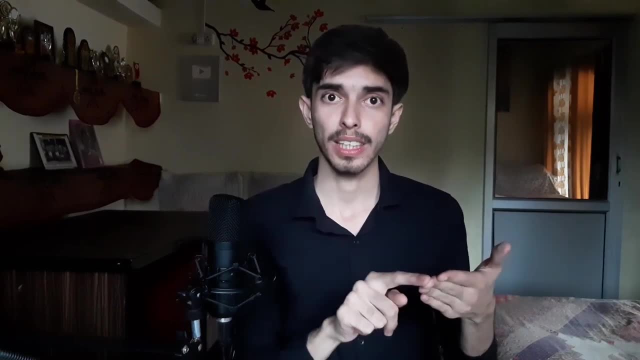 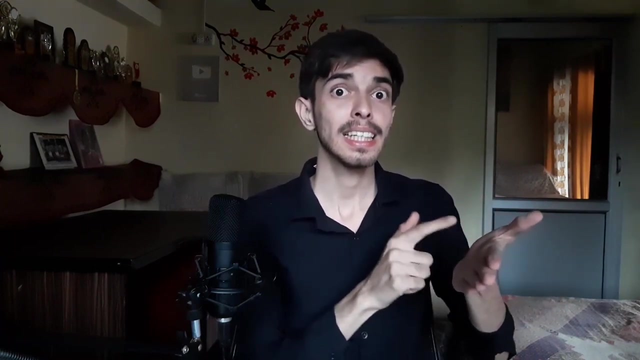 till 1600 there are zero odd days. okay, now we have to find for 43 years, and it is four years, so we will find the odd days till january 1643, so that 43th here is not yet passed. okay, so we will find the odd days till 31 december 1642 and then we will account for 4 january, as clear. so for 42 years, how many leap years are there and how many normal years are there? so divide it by 4, we get 10 leap years, and 42 minus 10 that means 32 normal years. for every leap year we have two odd days, so 20 odd days plus 32 odd days. add this up, we get 52. divide it by 7, we get a remainder of. 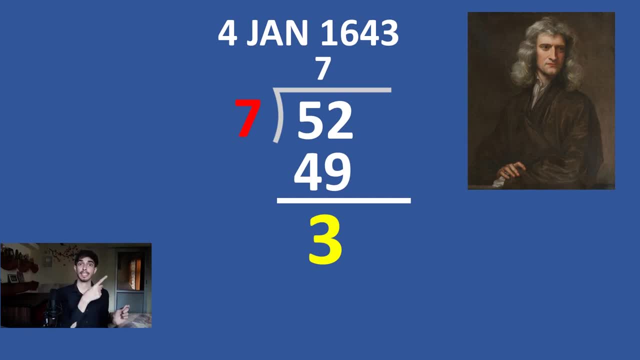 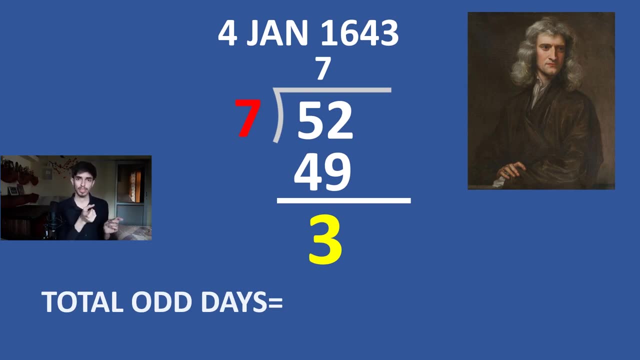 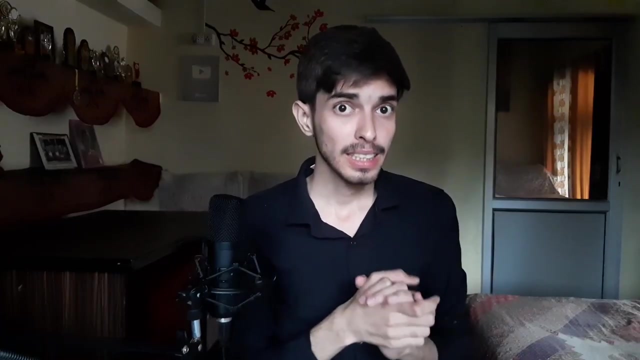 3. okay, so 3 odd days till 31 december 1642. now till 4 january we have 4 extra odd days because this is less than 7, so 4 days will count for 4 odd days. so 3 plus 4 is 7, so 7 is bigger than 6. 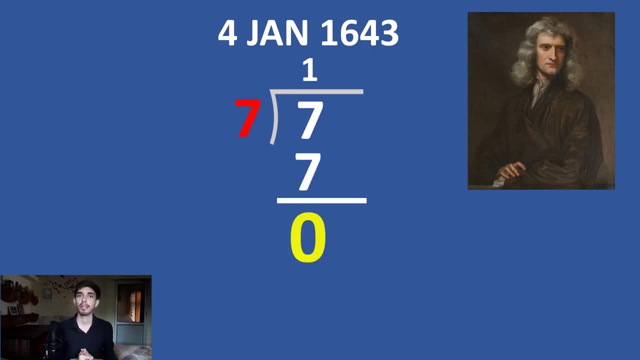 divide by 7 a remainder of 0. that means on the day of birth of sir isaac newton, we will find the date of birth of newton. it was a sunday, as simple as that. now let's calculate for 22 december 1887. 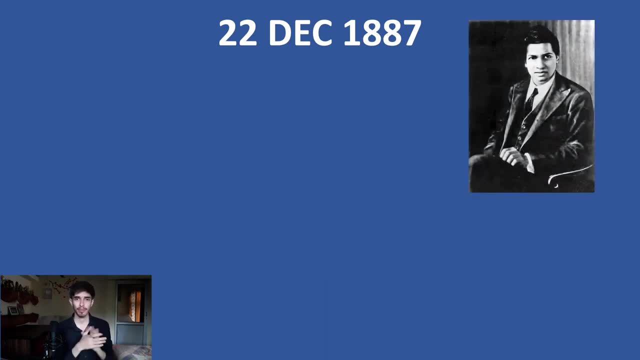 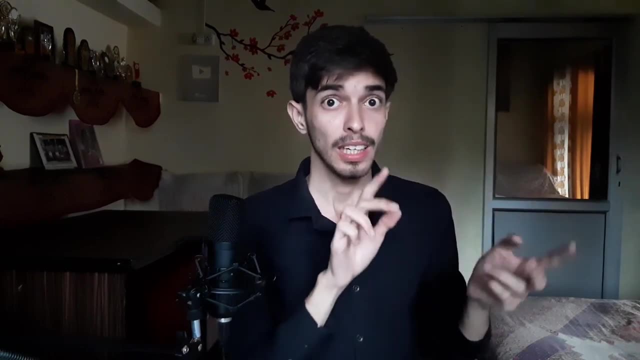 this is the date of birth of sri nivasana ramanujan. okay, we can do this with two different ways and you will learn two different techniques which are extremely important. so the second way is what i do not prefer, but in that there are some important techniques. so for this, what we can do is: 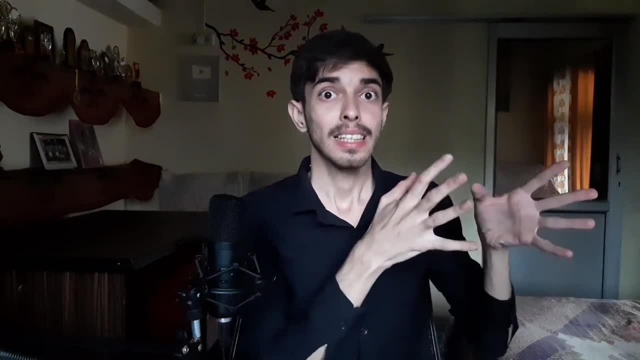 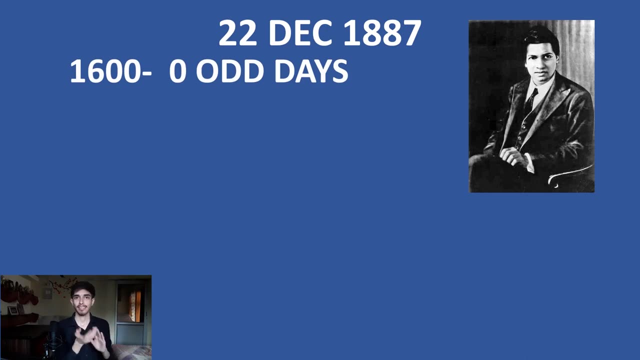 this, see, we can find the odd days till 31 december 1642, and then we will find the odd days till 31 december 1643, 1887, and go back nine days. as simple as that. so for 1887, see 1600, zero day, we have 200 more years. 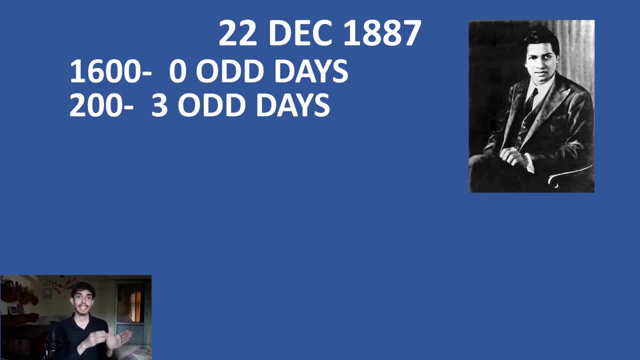 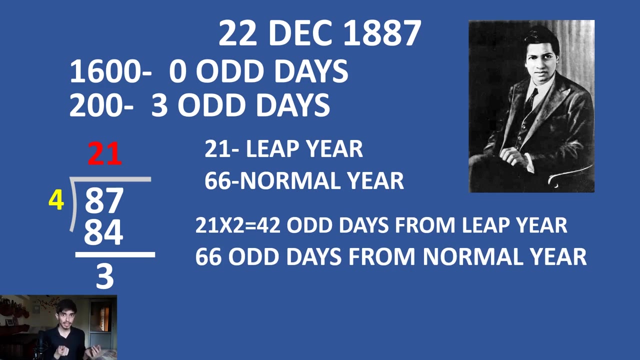 so three odd days. now we have to go till 87, okay, so divide it by four. with this we get 21 leap years and 66 normal years. from this we get 42 odd days from leap years and 66 odd days from normal years. add them up, we get 4 odd days till 31 december 1642, and then we have 2 odd days till 31 december 1643. 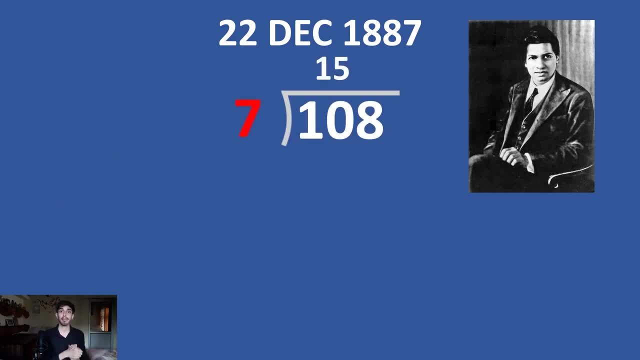 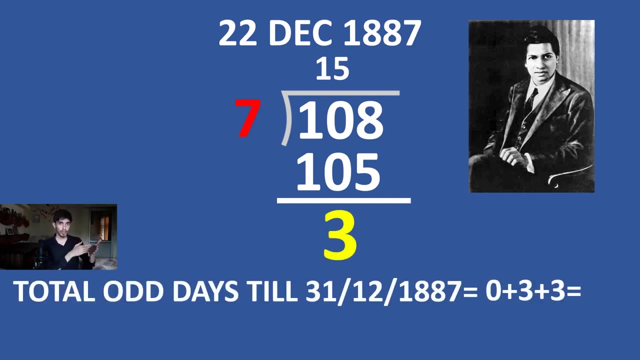 108 divided by 7 to get a remainder of 3, so till 31 december 1887 we have 0 from 1600, 3 from 200 years, and from 1887 we get 3 more so 6. so that means on 31 december 1887 we had a saturday, so now from 31. 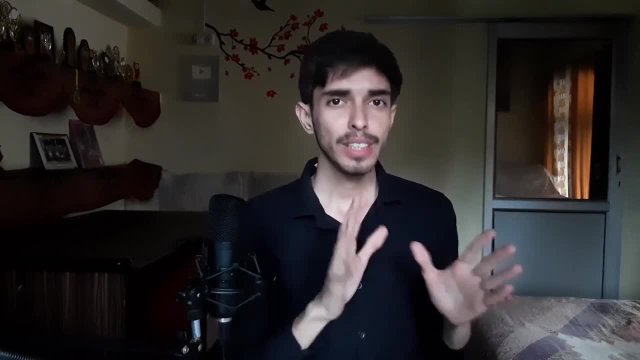 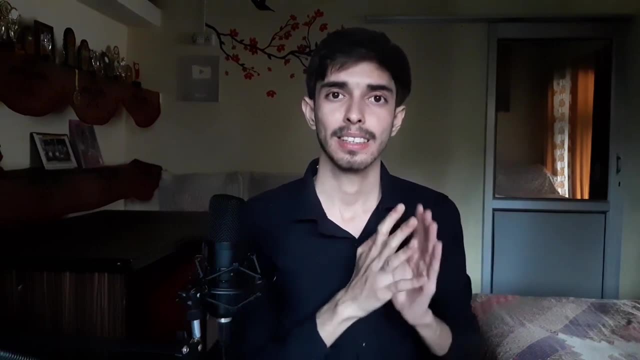 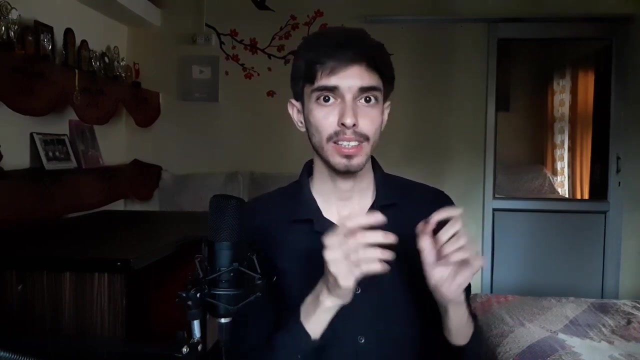 december to 22 december. we have to go back 9 days. we can do this in a more easy way. you can also go back like this, by just saying out the names. or you can do like this: see nine days, okay, divided by seven. so how many odd days? simple, two. so this simply means that we have counted two extra old. 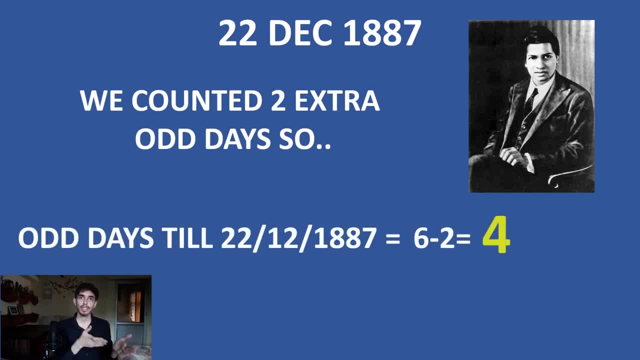 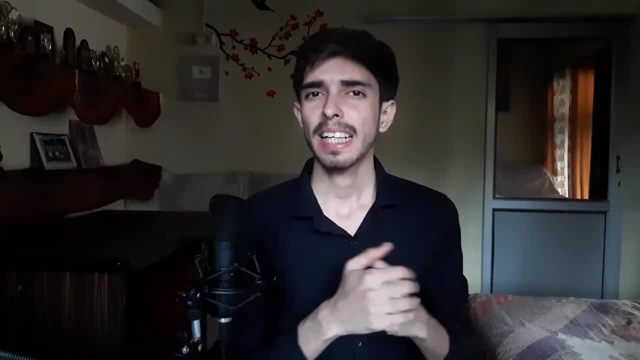 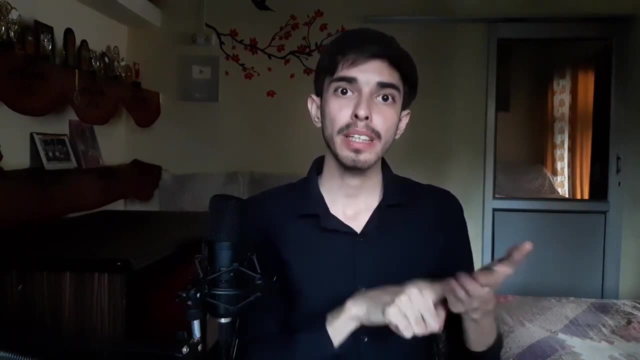 days, so subtract two from six, so six minus two, four, that means on the birthday of shri invasana ramanujan. it was a thursday. and the second way is this: we can count the odd days till 31 december 18, 86, and then, month by month, by month, we can count the odd days and go till 22 december 1887. let's do. 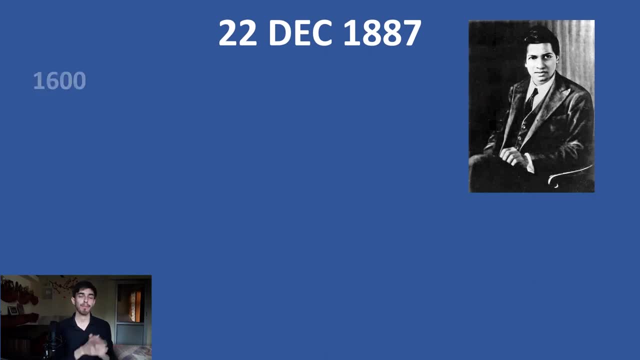 it. it is extremely simple: till 1886, see till 1600 zero days, 200 more years, three odd days now for 86. i am sure now you can calculate the odd days. the odd days for 86 years is two. this is an exercise that you can do. you will get two odd days for 86 years, okay. now we have to go month by month by month to our required date. so first january: we have 31 days in january, so san forza 28, so we have three odd days now in february. it is 1887, right, not a leap year. 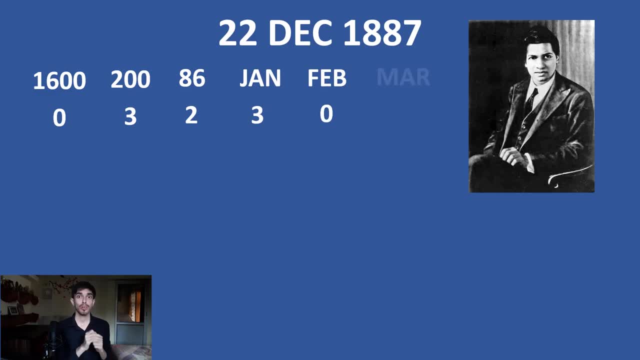 so we have 28 days. that means zero days. for march, we have three odd days. for april we have two odd days, and so on. we calculate till november, and then for december it will be two odd days, and then for en ausent voted by seven, we get one odd day. add these all up, we get thirty two divided by seven.